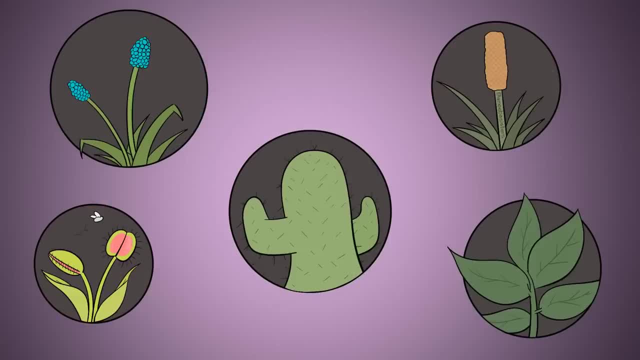 different types of animals. Well, there are many different types of plants as well. They don't all require the exact same amount of light and the exact same amount of water. There is so much diversity in plants. There are over 300,000 estimated species of plants. 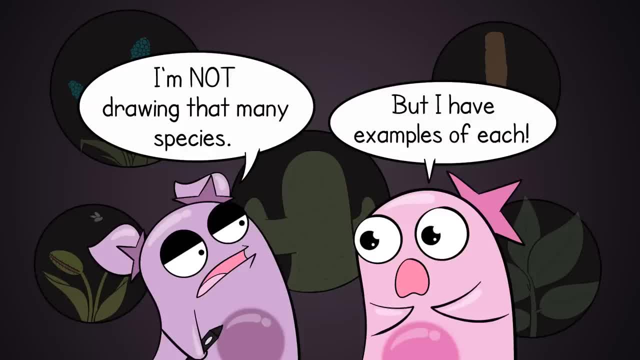 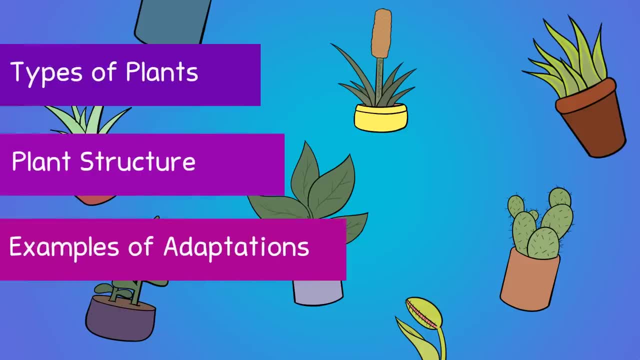 And there are some fascinating adaptations that have helped them live in a variety of environments. This video is going to briefly touch on types of plants, their structure and some fascinating adaptations. First, we need to outline two general plant categories: vascular and nonvascular. Recall in the human body, your 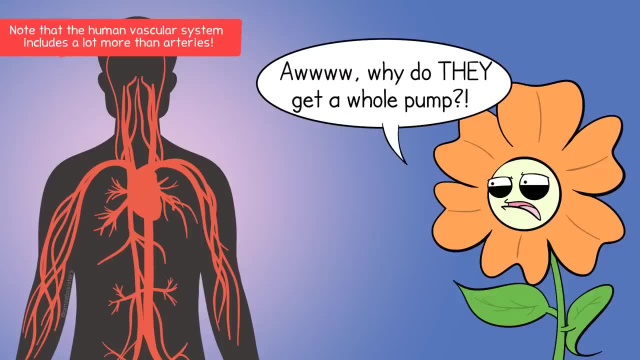 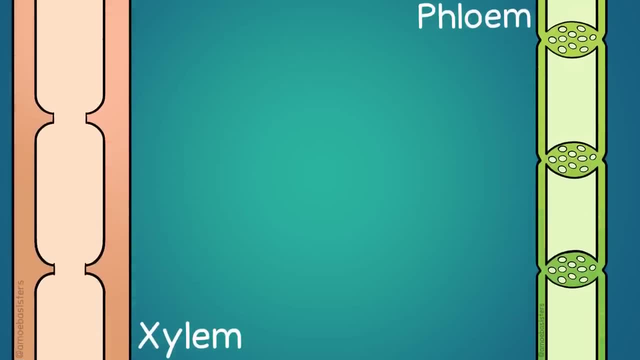 vascular system includes arteries. Well, plants don't have arteries, or blood for that matter. When we're talking about a vascular system in plants, we're talking about two major types of tubes or vessels called the xylem and phloem. The xylem carries water, The xylem 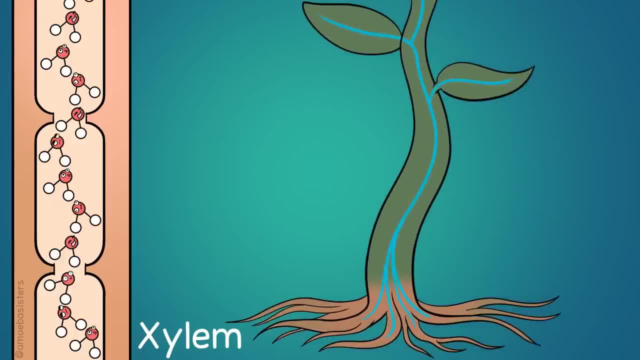 is found throughout a vascular plant. Water is absorbed from the roots of a vascular plant and carried upwards. Roots help anchor plants and also absorb the water found in the soil that they are in. The xylem continues up from the roots through the stem to the leaves. Structure-wise, the 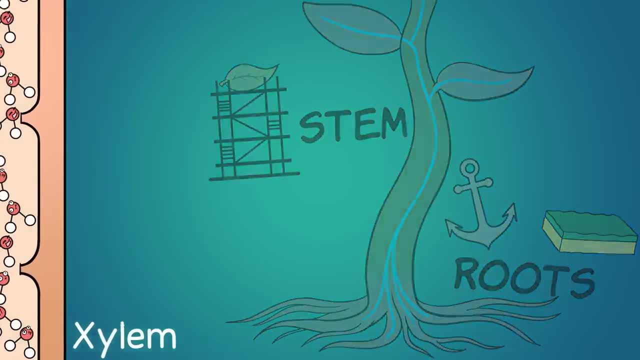 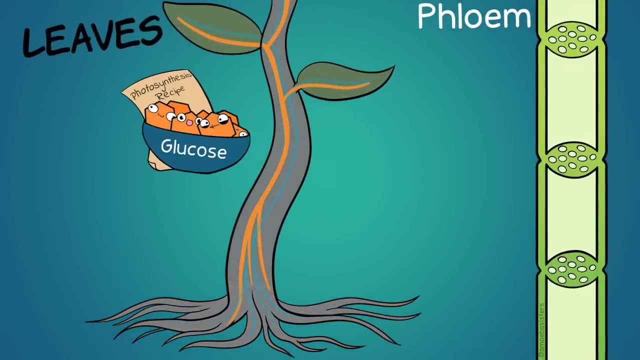 stem has a function of providing support to the leaves, Now the other vascular tissue, the phloem. So recall that glucose, a sugar, is typically produced in the leaves during photosynthesis. All the plant cells will need sugar. Sugar is the plant's food source. 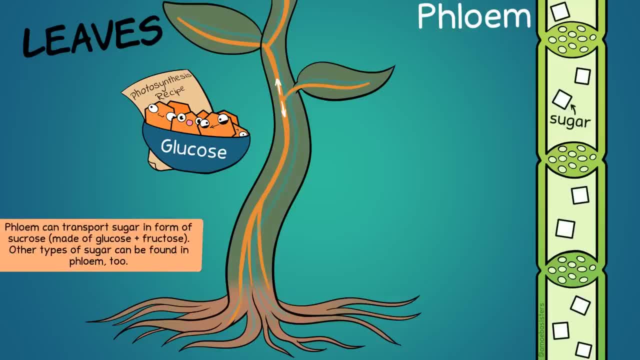 The phloem carries sugar from the leaves, where it's generally made throughout the plant. By the way, the word phloem might start with a P, but it does have the same F sound that food has, So it helps me remember that it carries the plant. So phloem is the plant's food source. The phloem is the plant's food source. The phloem carries the plant's food. The phloem is the plant's food source. The phloem is the plant's food source. The phloem carries the plant's food. 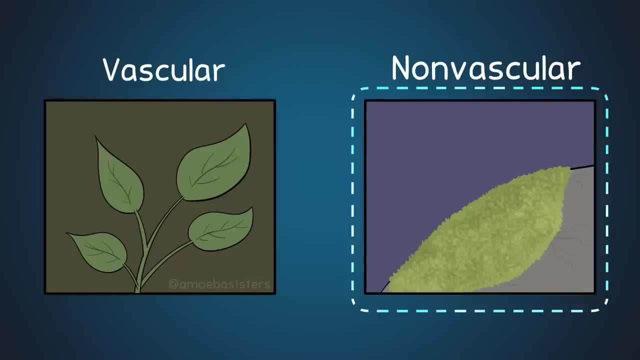 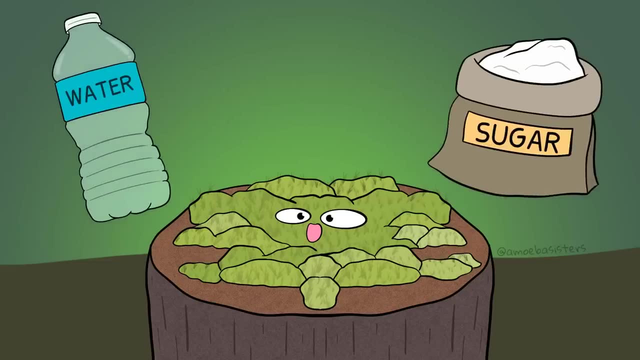 If a plant is non-vascular, it does not have vessels like the xylem and phloem. However, it still needs water and it still produces sugar. It just can't carry it upwards in the xylem because it doesn't have one. 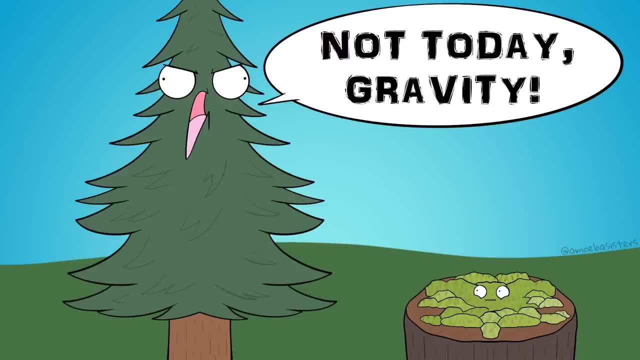 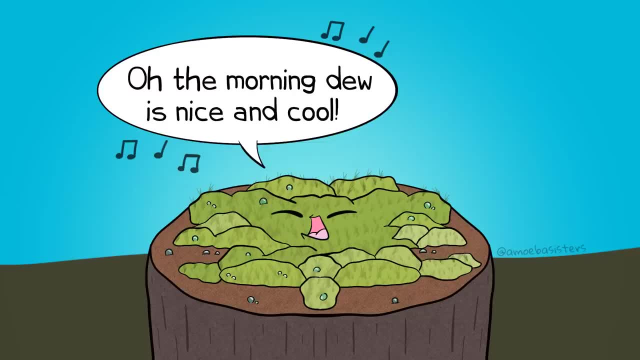 That means non-vascular plants typically are limited in size. A giant tree needs a xylem for water transport. The water is being carried against gravity. Non-vascular plants instead get their water by osmosis, Kind of like soaking up water like a sponge. Non-vascular plants. 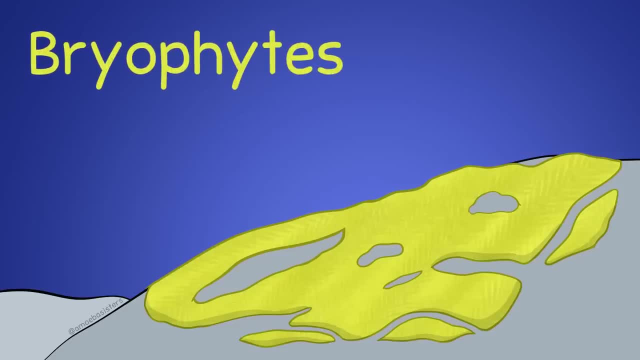 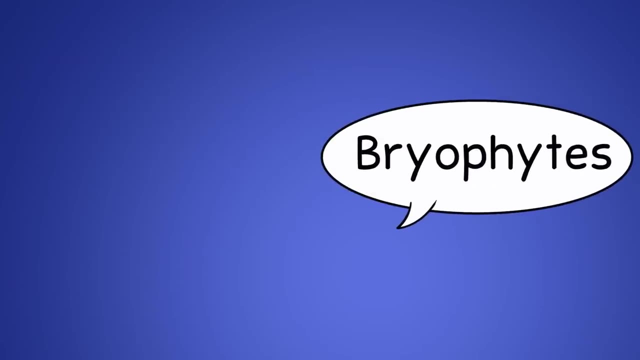 are often informally called phloem, called bryophytes. I say informally because it's kind of like when you use the informal word protist. The term bryophytes is often a collective informal term that includes three different phyla. 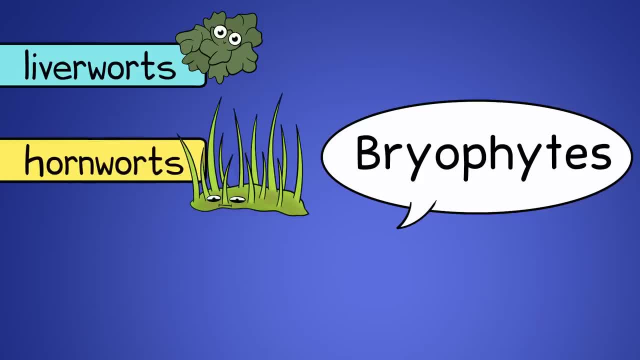 A phylum that contains liverworts, a phylum that contains hornworts and a phylum that contains mosses, And actually the phylum that includes mosses is a phylum called bryophyta. So again, 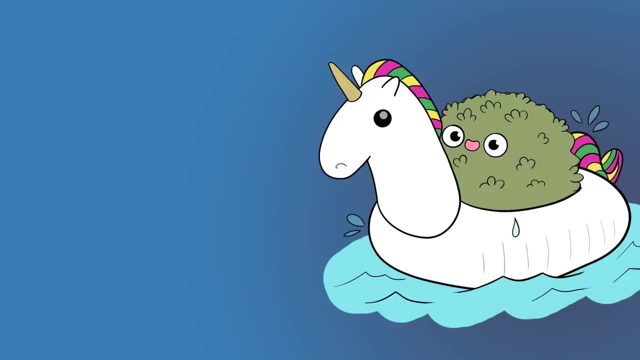 just be aware of the informal use of the word bryophytes, As they're nonvascular. bryophytes are generally small and are more frequently, but not always, found in areas where there's a lot of moisture. They do not have true stems, nor true leaves, nor true roots. 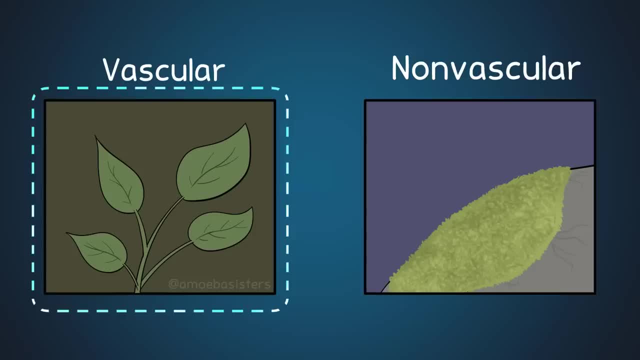 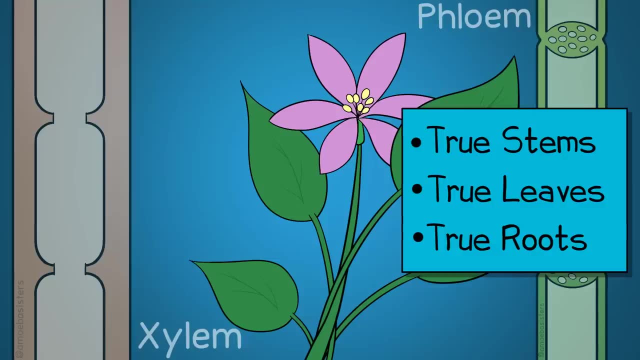 although they can have structures that resemble them. Now let's briefly discuss vascular plants. Again, vascular plants have xylem and phloem. These plants have true stems, leaves and roots. We can arrange vascular plants into three general categories. The first category: 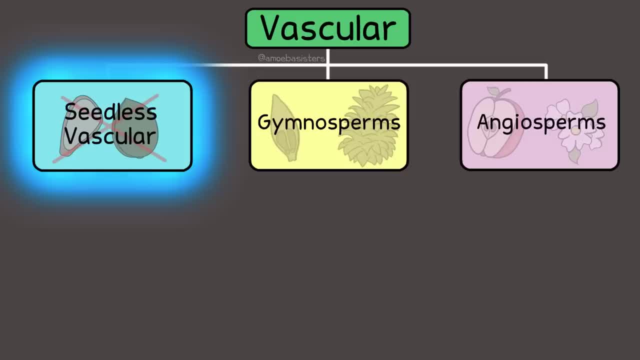 seedless vascular plants. As their names suggest, they have no seeds. This group includes a phylum, a phylum and a phylum. The second category is the seedless vascular plants. This includes a phylum that contains lycophytes like club mosses, which are different than the. 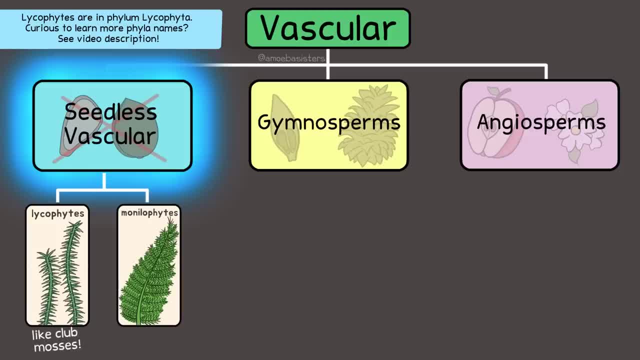 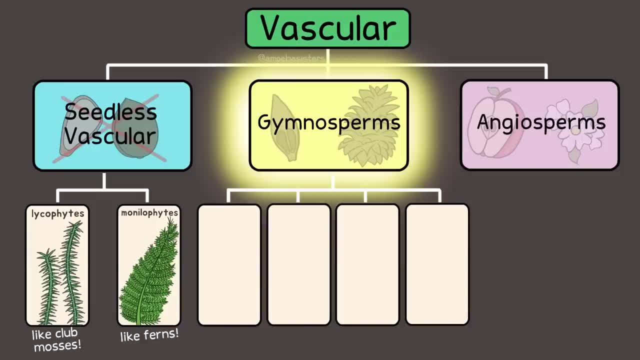 moss and the bryophytes, And it includes a phylum that contains monilophytes like ferns. Second category: gymnosperms. These include several phyla: one phylum that has ginkgo, one phylum that has cycads, one phylum that has neidophytes and one phylum that has conifers. 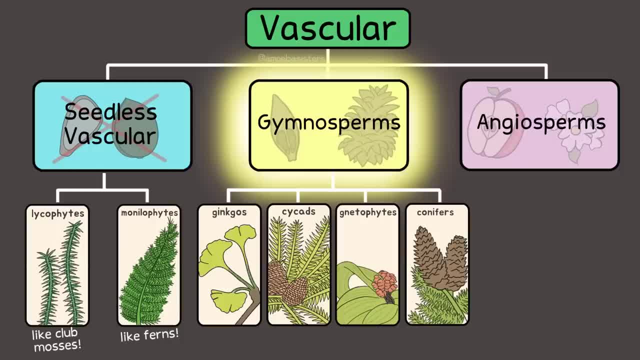 The word gymnosperm means naked seed, as they don't have their seeds enclosed, like the next group will get to. Instead, many gymnosperms have cones. Gymnosperms have neither flowers nor fruit. Third category: angiosperms. These are the flowering plants. They have flowers. 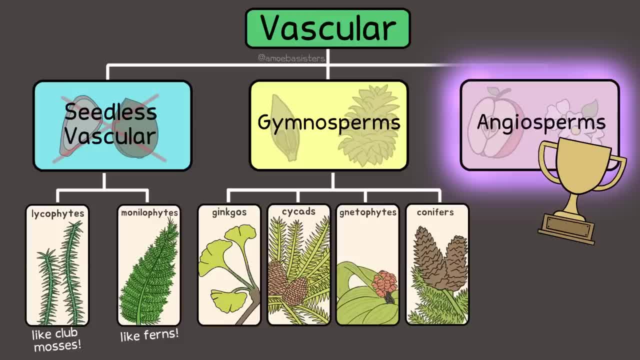 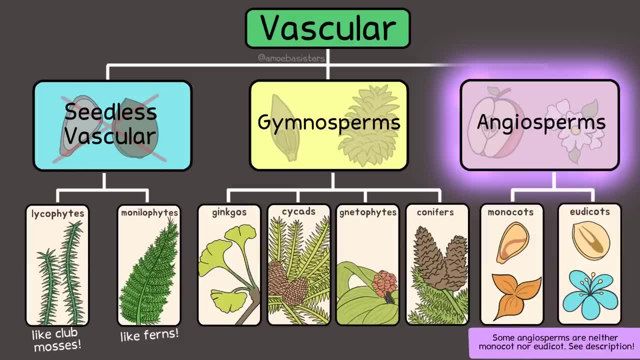 they have fruit, though not necessarily an edible fruit. This is a huge group. It's estimated around 90% of all plants are angiosperms Within the angiosperm group. many angiosperms, but not all, can be categorized as a monocot or eudicot. 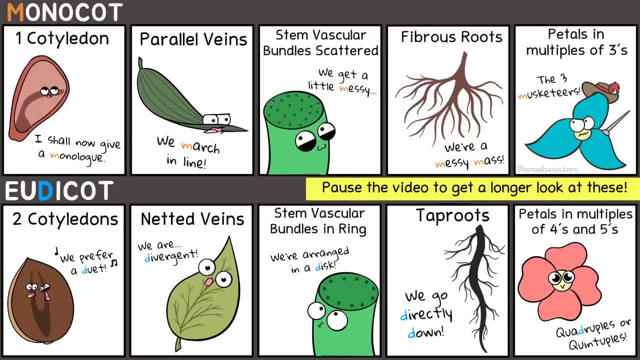 You'll see some of the characteristics we included of these two groups in our illustrations here. But first let's look at the angiosperm group. But just know there are some exceptions. Overall, just trying to really emphasize, the angiosperm group is the largest, most diverse group of plants. 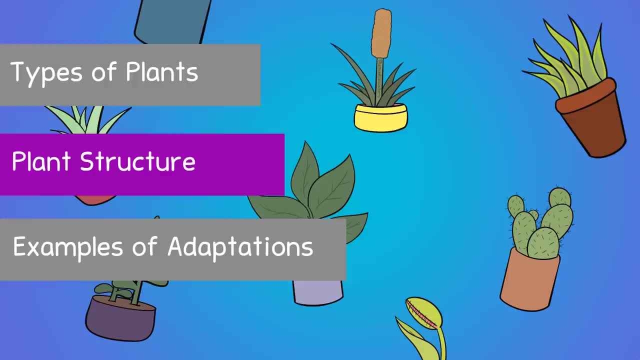 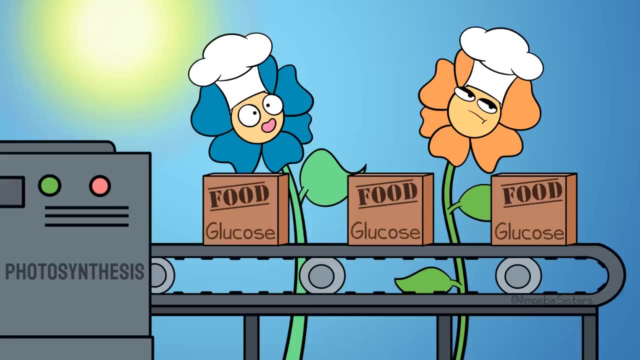 Even though every plant species is unique, let's talk about general plant structure. The structure of plants is critical for plants to be able to perform photosynthesis. Photosynthesis is the ability to make sugar, the plant's own food source, from sunlight. 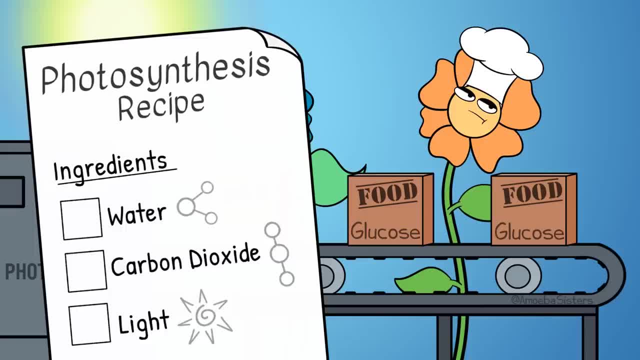 And it requires three main ingredients- water, carbon dioxide and light- To get all three of these things. the plant needs specific ingredients. To get the right amount of water, the plant needs specific ingredients To get the right amount of water. the plant needs specific ingredients To get. 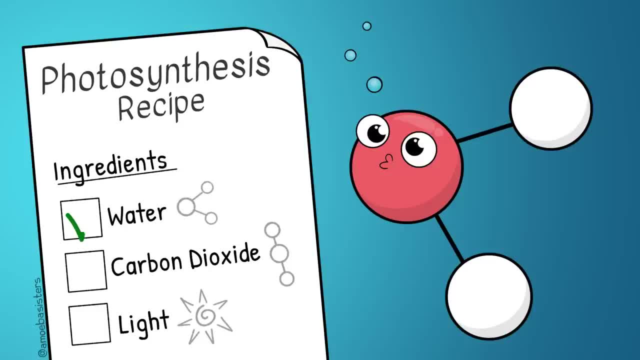 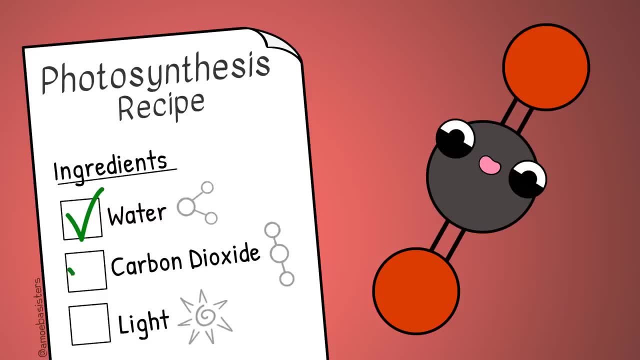 the right amount of water. the plant needs specific structures and adaptations, which we're going to walk through. First water: We mentioned already how a plant can obtain it in different ways depending on whether they're vascular or nonvascular. Next, carbon dioxide. Many plants have these fascinating little openings- pores, really. 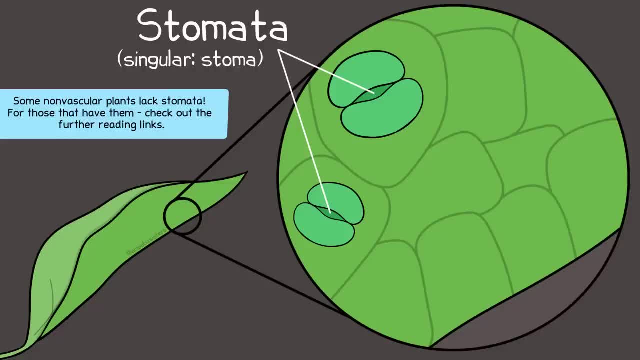 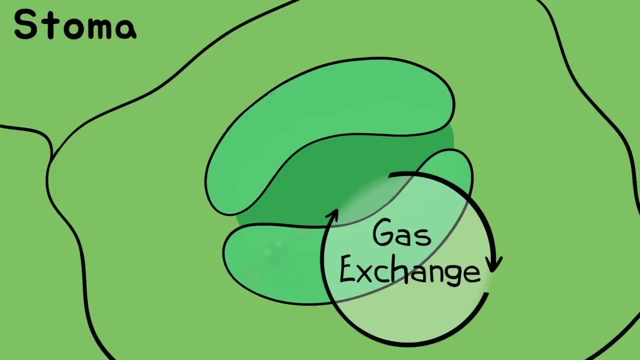 called stomata or singular stoma. Stomata are typically, but not always, found on the bottom of leaves. Stomata have a major role in gas exchange because gases can travel through them And a gas plants need directly for photosynthesis is carbon dioxide. 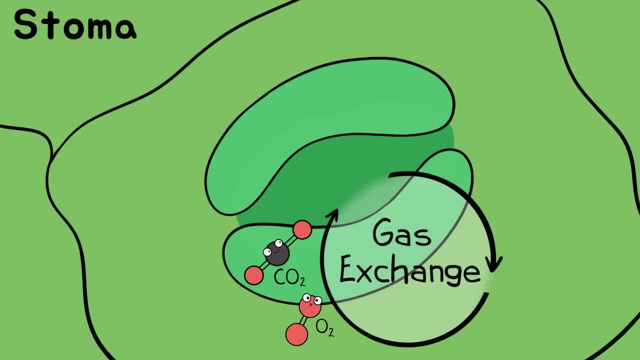 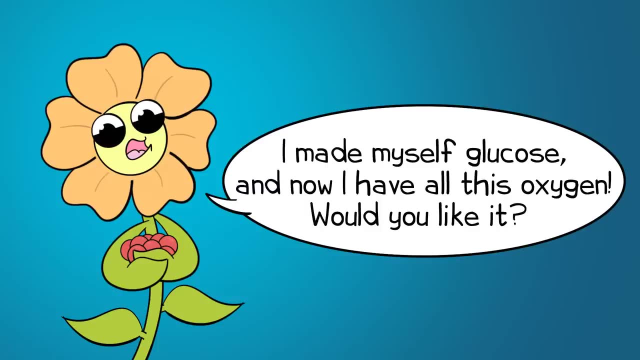 But don't forget when it comes to gases. plants also do cellular respiration, And to do that they need the gas oxygen. However, plants generally produce more oxygen in photosynthesis than they need in cellular respiration. Now, while gases can flow in through these stomata, 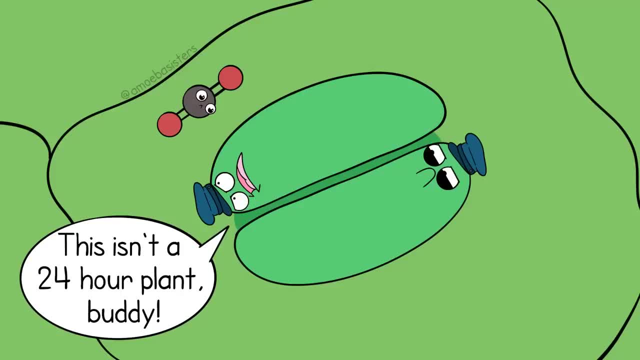 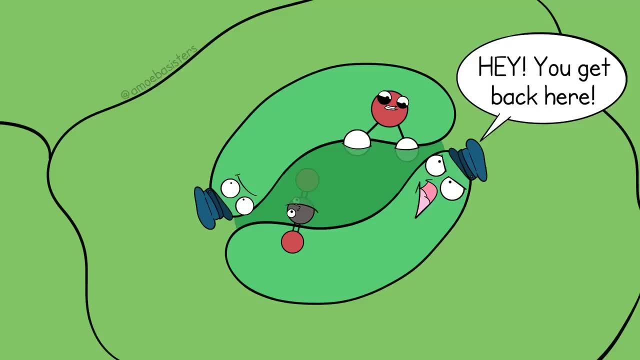 there's still a little problem. Plants can't usually keep those stomata open all the time. When they're open, water can escape And, remember, plants need water too for photosynthesis. So the plant must determine whether to open or close its stomata, And it does this with the help 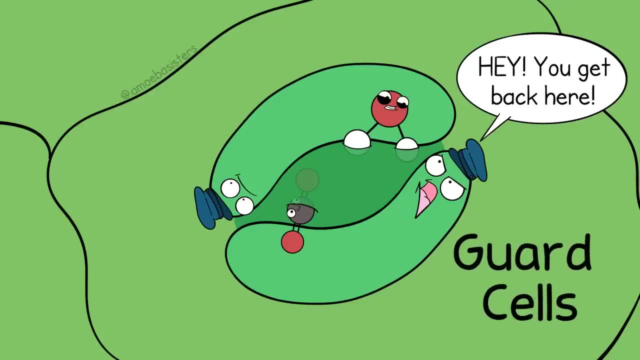 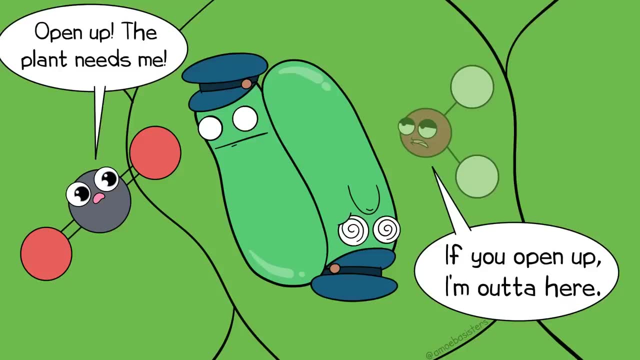 of guard cells. If guard cells have the stomata open, the plant gets the gases it needs But it can lose water. If guard cells have the stomata closed, it gets to save its water but then it limits gas exchange At night. many plants, with a few exceptions. 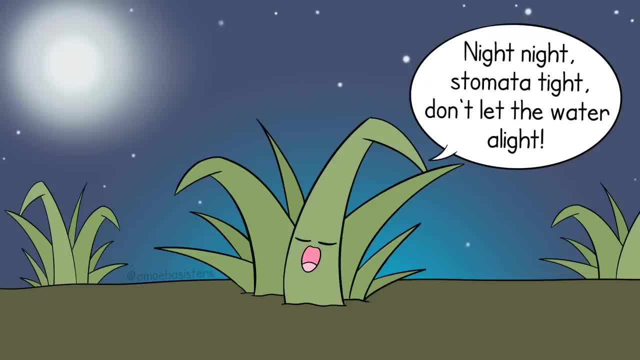 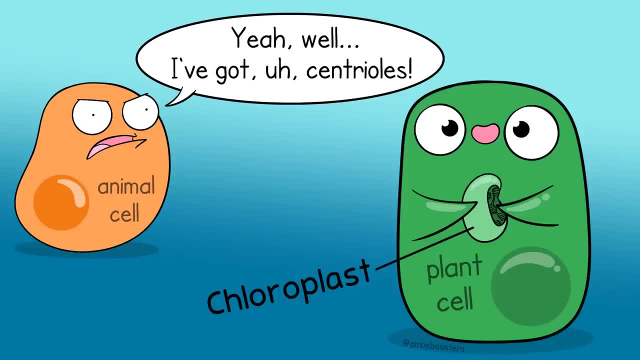 close their stomata so they can conserve their water, as they aren't doing photosynthesis at night. Last on the list that plants need to capture is light. Plant cells have organelles called chloroplasts. These amazing organelles are not found in animal cells. They are the site of 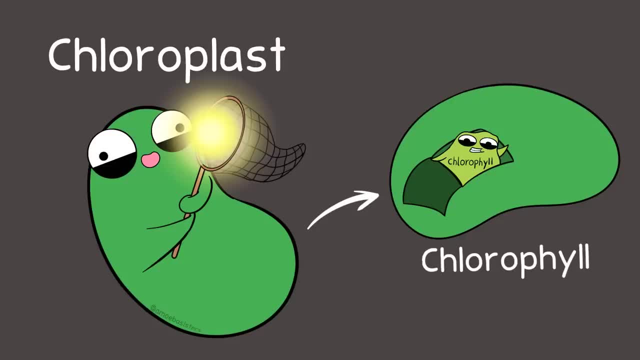 plants, so they help capture light energy for the process of photosynthesis. Plants also have pigments there. Chlorophyll is a major one that can absorb certain wavelengths of light like red or blue light. But plants can contain other pigments too, which can expand the different 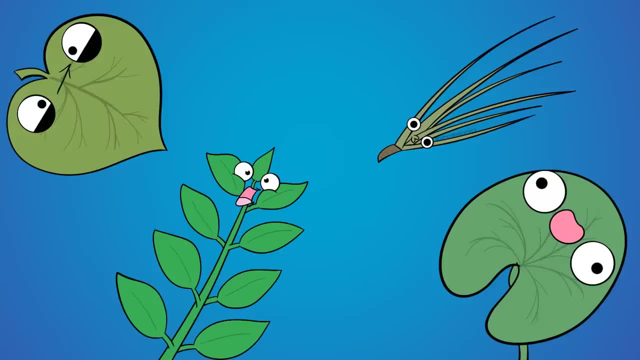 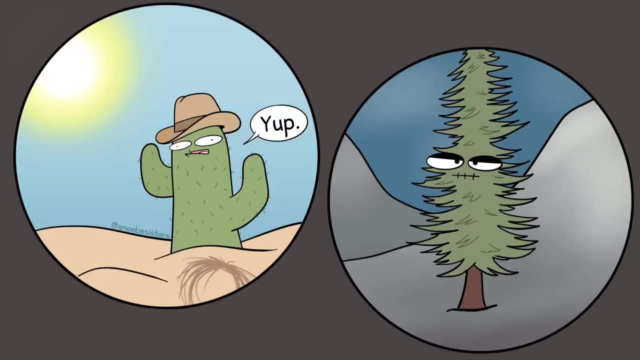 wavelengths of light that they absorb. Leaf structure is really important when it comes to capturing light energy. The size and shape of leaves can be different based on where different species are found. Plants that live in areas where they must conserve water might have thin leaves. 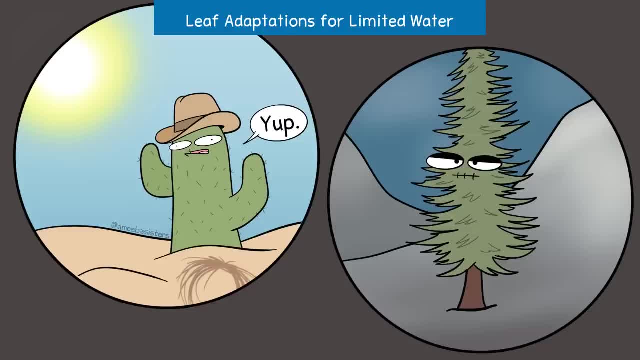 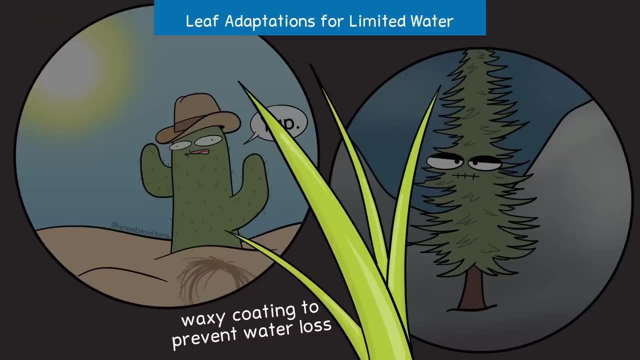 so they don't have much surface area to lose water. Plants that don't have much surface area to lose water- Think about pine trees with their skinny pine needle leaves, or think about plants that live in the desert. Many of these plants also have especially waxy leaf cuticles to protect. 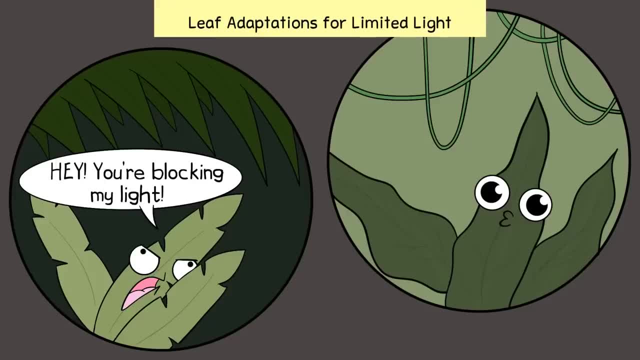 against water loss through the leaves. Plants that have lots of access to water but maybe are shaded by a lot of taller plants in the jungle might have really broad, wide leaves so they can soak up as much sun as possible. It's hard to live in someone else's shadow, Since there is plenty of. 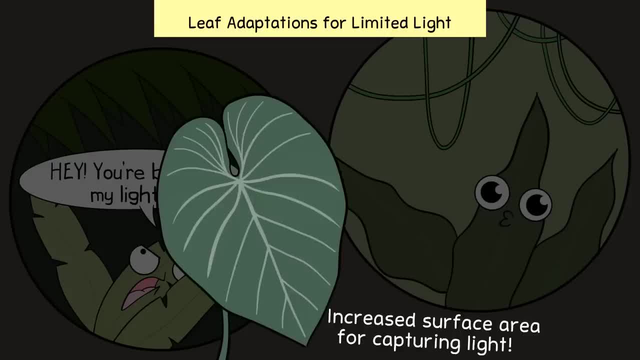 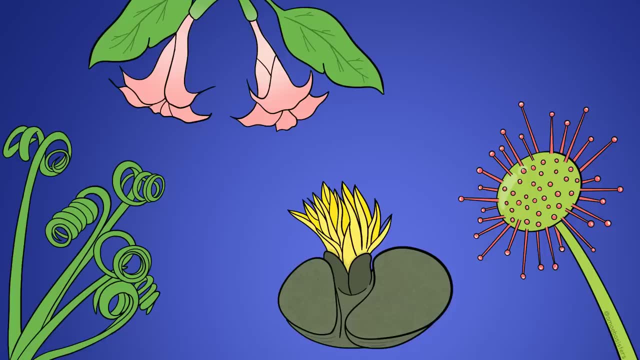 water. these plants may not struggle with water loss concern and can have more leaf surface area. We talked about general plant structure, but obviously there are plants all over the world with unique structures and adaptations. Before we end our video, we want to conclude with some 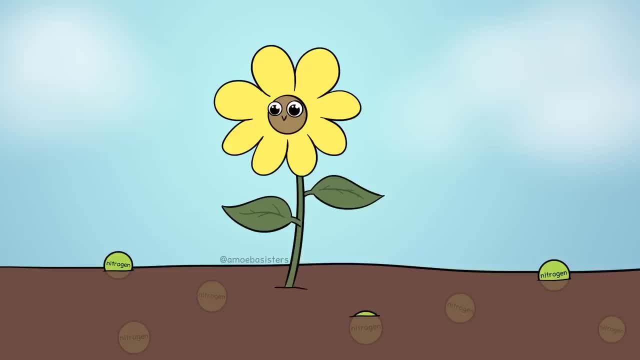 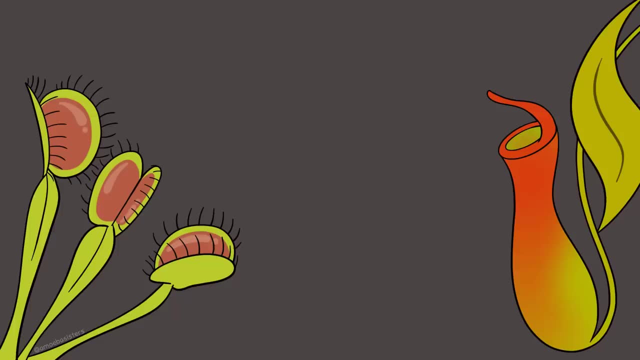 especially fascinating ones. Plants and other organisms use nitrogen in the building of proteins. So what happens if plants live where the soil is low in nitrogen? You may have heard of carnivorous plants like the Venus flytrap or the pitcher plant. These plants still do. 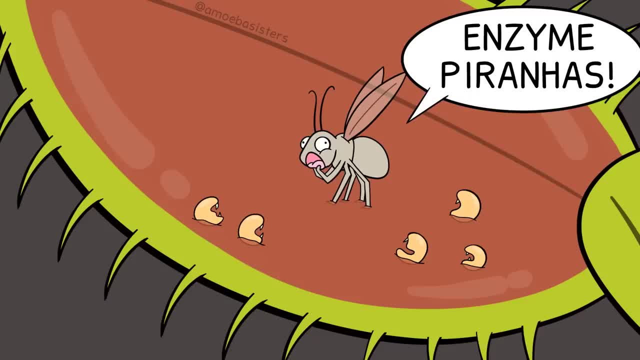 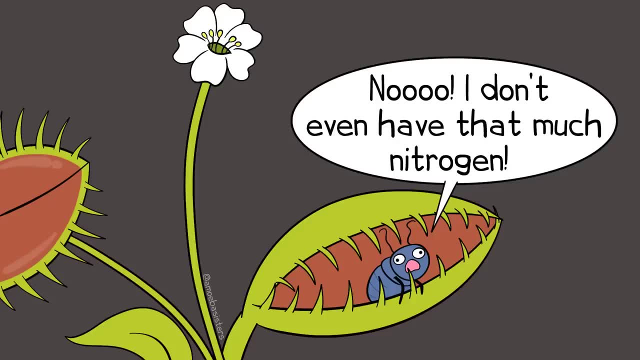 photosynthesis to make their sugar. but carnivorous plants also have the ability to digest insects, typically by using special enzymes in a juice they secrete. Insects are a great way to supplement their nitrogen need. If you ever look at ingredients in plant fertilizer, you will find 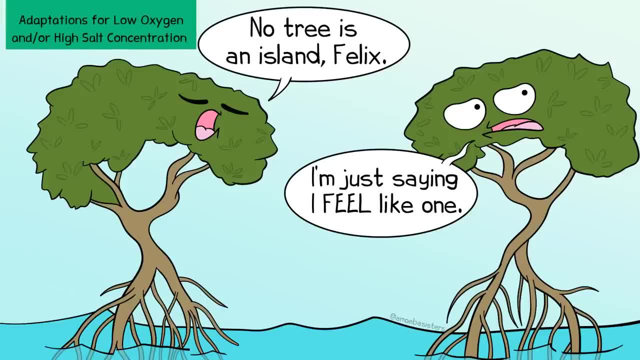 many fertilizers are high in nitrogen. You can also have too much of a usually good thing. What about plants that live where it's too wet? Many types of mangrove trees live in waterlogged soil. These plants can have specialized roots that help them deal with the low oxygen. 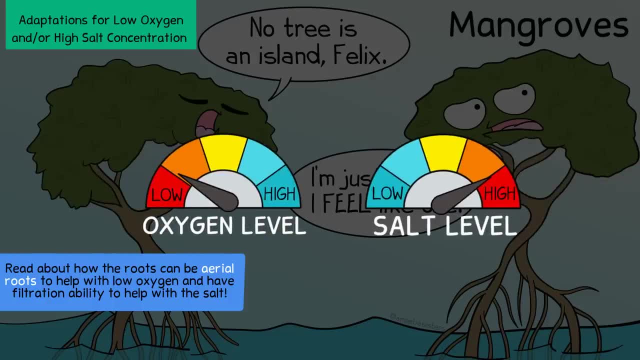 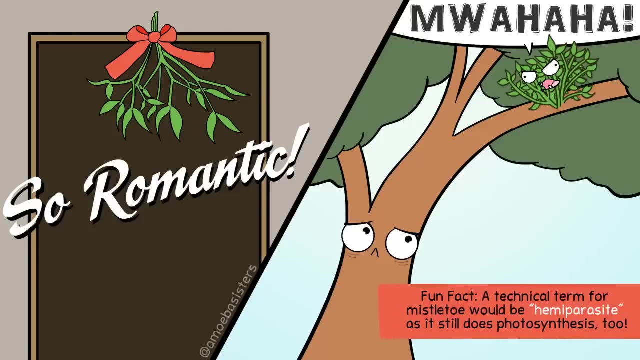 and potentially high salt concentrations in a variety of ways. see our recommended reading. Plants can even turn into thieves to get the nutrients they need. You've heard of mistletoe. Is it terribly ironic that they can be parasitic if they can use their specialized roots to steal?